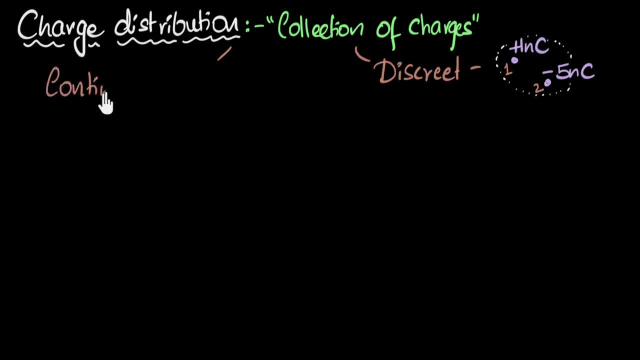 This is called continuous charge, distribution Continuous. And let me immediately give you an example of that. So let's say we have a wire And let's imagine I charge up this wire And let's say it gets a positive charge. So now the positive charge. 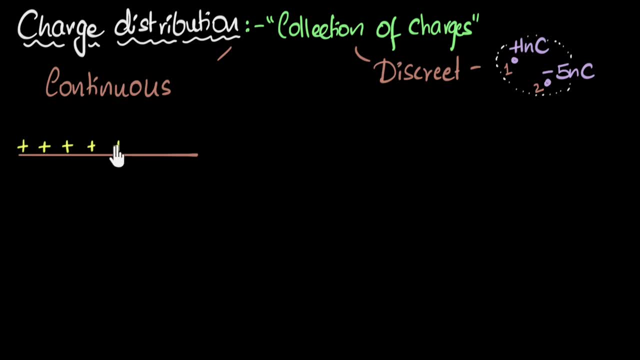 will be continuously spread along this wire. Now, I don't mean that there is a charge here and then there are no charges in between and there is a charge here. That's not what I'm saying. What I'm saying now is the charges are spread out. 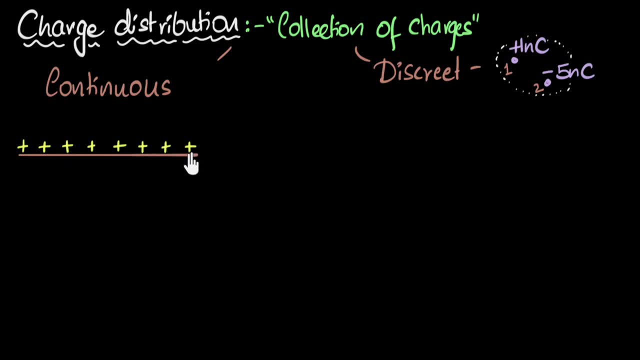 There's charge everywhere. This is what we call a continuous charge distribution. And do you know what's interesting about this? I can have that same wire and I can have that same amount of charge. Let's say this total charge is- I don't know. 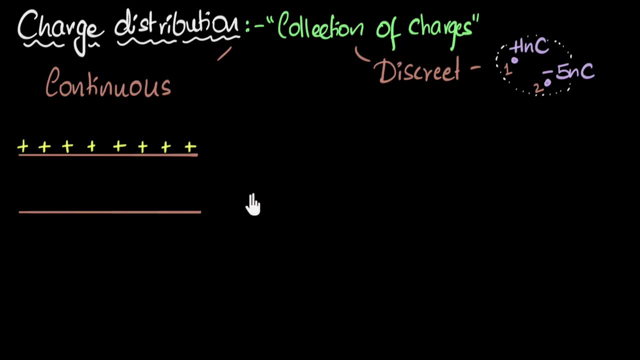 maybe 100 coulomb, and I can distribute it continuously in a different way, For example. you know what I can do. I can distribute it maybe somewhat like this. Now again, I don't mean that there are no charges in between. 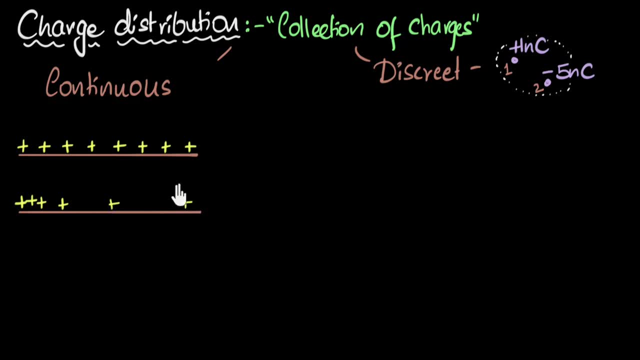 It's a continuous distribution. There are charges everywhere, And so the total charge here is the same as the total charge over here. But what's the difference? Well, the difference is the charges are more crowded over here and they are less crowded over here. 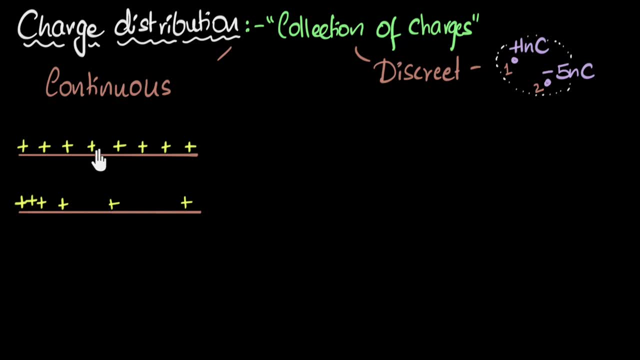 That's what I'm representing. But over here the charges are equally crowded everywhere, And that's why, when we're talking about continuous charge distributions, this is an important quantity: How crowded the charges are. Are they uniformly crowded everywhere, or are they more crowded at one place? 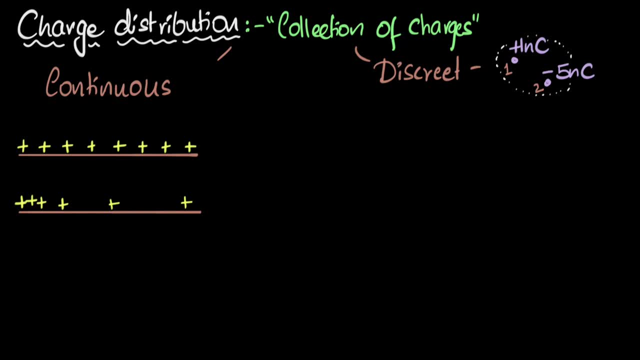 and less crowded at some other place. And that's why, when it comes to continuous charge distribution, we introduce a new quantity called charge density. You may have heard of the word density. The word density- sorry. The word density basically means how crowded something is. 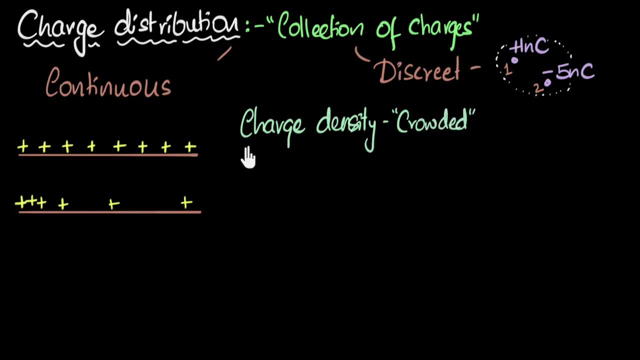 So when we say charge density, we're talking about how crowded the charges are, And when we're dealing with charged distribution over a line- and we'll talk more about different kinds of distribution in a minute- Whenever we're dealing with that, the symbol that we use to 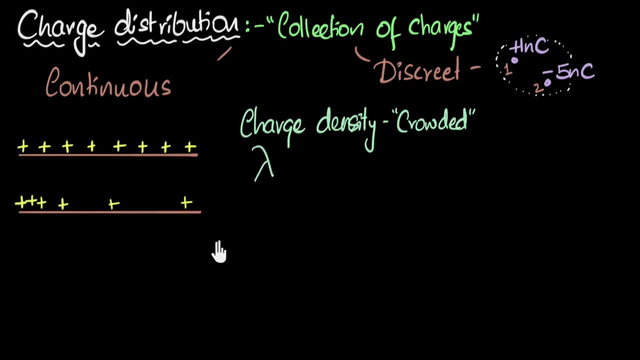 charge density is the Greek symbol, lambda, and this number basically tells you how crowded the charges are or on a given length. and so the way we represent lambda, or with the way we calculate lambda is we say how much charge is present over unit length, and I'll give you an example. but before that, let's 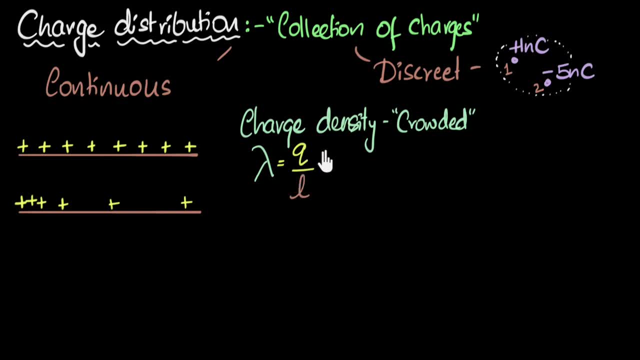 talk about the units. what would be the units of charge density? well, the unit of charge density would be coulomb per meter. so, for example, I could say: hey, the charge density over here for this, this wire, is 20 coulomb per meter. what does? 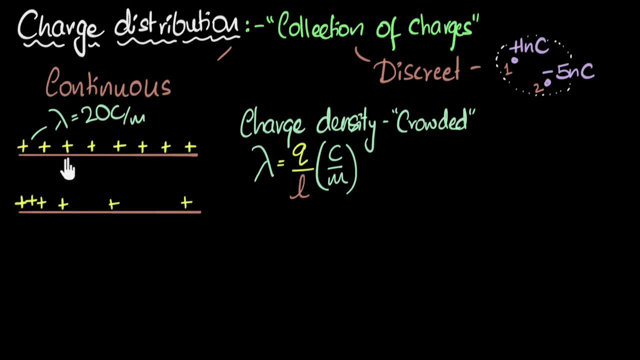 that mean? that means if I were to take one meter of this wire- and I don't know how long this wire is, but let's say it's a very, very long wire- and I took one meter of this, in that one meter I would find one meter of this wire. and I took one meter of this, in that one meter I would. 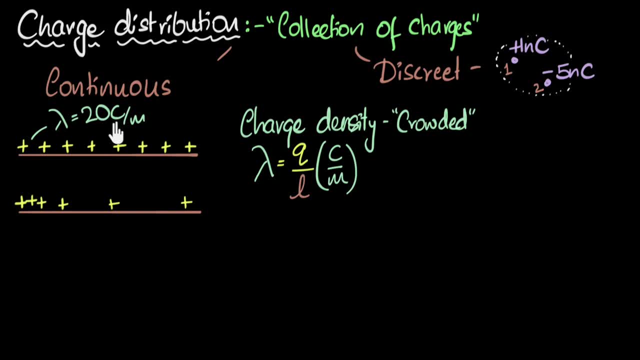 find 20 coulombs of charge. that's what this means, and I can take that one meter anywhere and I'll find 20 coulombs. the charge density over here is a constant because it's equally crowded everywhere. so what if I take two meters of length? 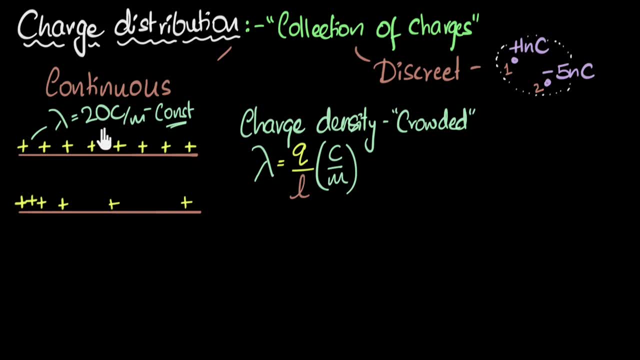 how much charge would I find over there? well, per meter is 20, so in two meters I'll find 40 coulombs of charge. if I take a half a meter, how much charge would I find over there? well, I would find 10 coulombs of charge. does this make sense? you understand what charge density. 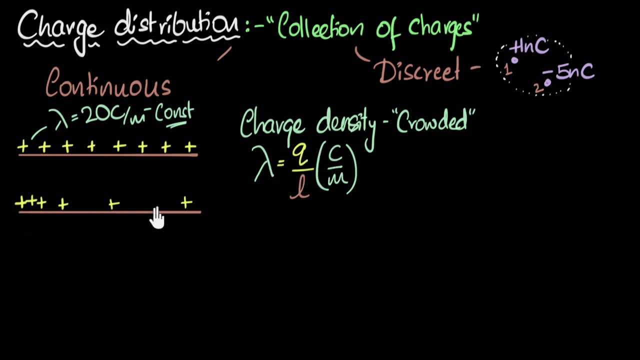 is okay. what about charge density over here? can I give one number for charge density over here? no, because the charge density varies. you have a. you can kind of say it's a very high charge density over here, there is very low charge density over here, and how do I represent that? how do I figure? how do I give a? 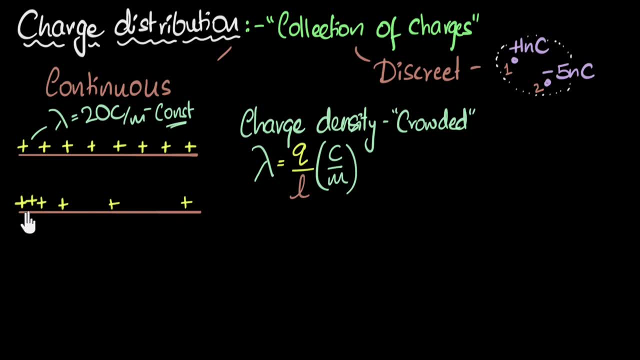 number to it. the way to give a number over here is you could say you could take a very tiny, very tiny length and let's say that length is I don't know, maybe a nanometer. okay, take a very, very tiny length and in that length find out how many charges. 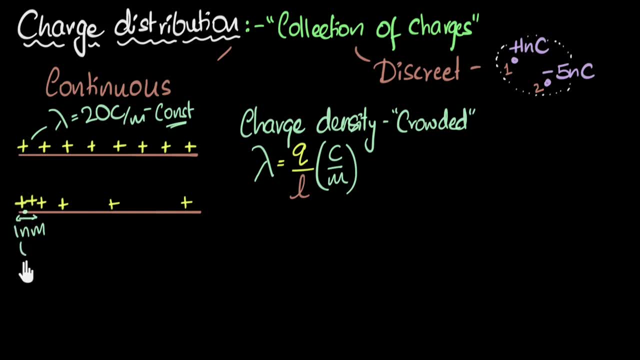 are present, maybe in that one nanometer, I find I don't know- maybe 50 nano coulombs of charge. now I will say at that point: lambda, which is our charge density, is 50 nano coulombs divided by one nanometer, so that would be 50 coulomb per meter. 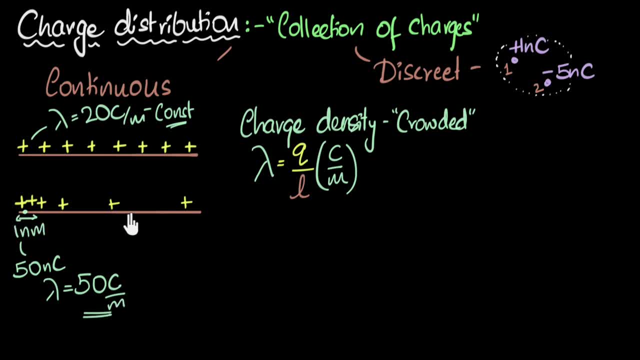 and now what's interesting is, this does not mean I take one meter and I'll find 50 coulombs. no, this basically says: at that point you will find. if you take the charge and divide by length, that ratio turns out to be 50. so this is the value. 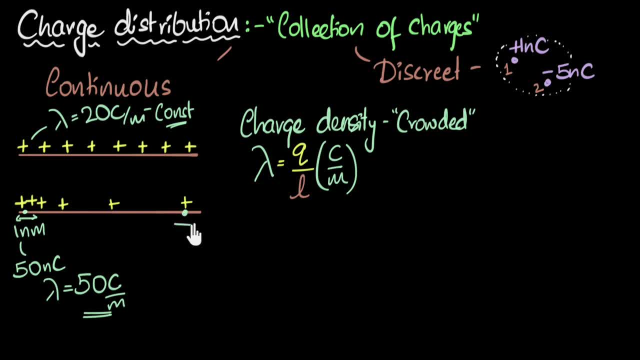 at that point. similarly, if I were to take- maybe at this point I take one nanometer over here and I'm just using nano as an example- you imagine it's a very incredibly tiny, tiny point. you know tiny distance you're taking in that one nanometer. maybe I'll just find only two nanometers. maybe I'll just find only two. 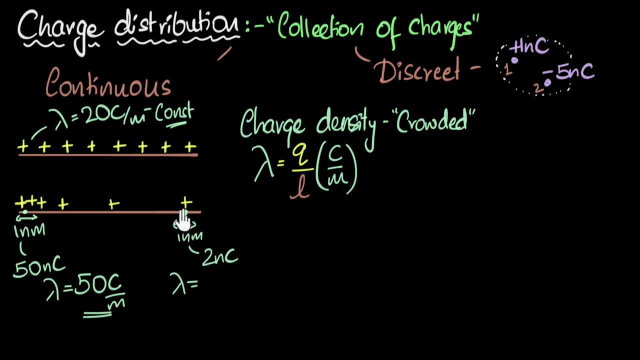 nano coulombs at this point. so we will say: the lambda at this point would be two nano coulomb divided by nanometer, it'll be two coulomb per meter. so over here, how do you calculate charge density? well, we calculate charge density lambda by: 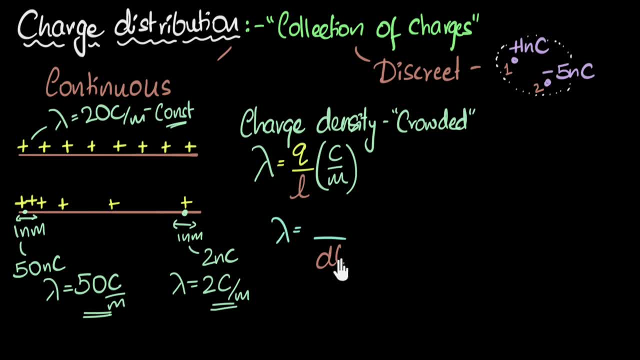 taking very tiny lengths, DL. that's how you write it mathematically, even though I've shown using like real numbers over here. but mathematically it's an infinitesimal length you take and over that you find how much charge is present and that ratio tells you the charge density at. 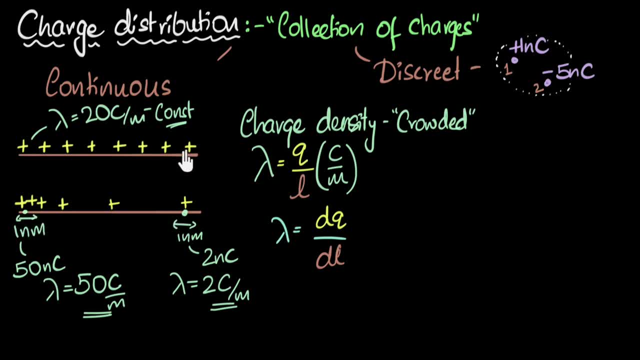 individual points. so if the charge is uniformly distributed, then whether you take it at a point or you take it over a large length, that value stays the same, and that's pretty much about charge distribution. but now you could ask, wait a second. here charges were distributed over a line, and so we like to call this. 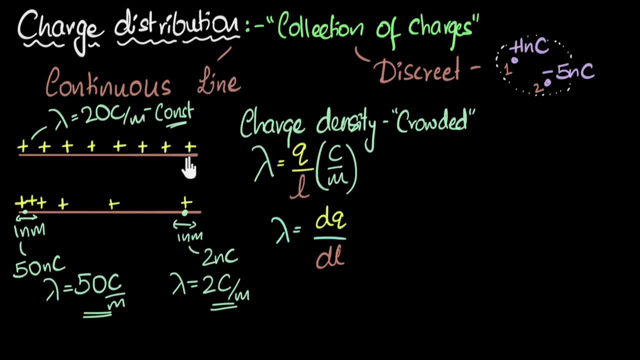 a continuous line charge distribution and therefore this density we like to give it a name. we call this linear charge density because it's telling you how much charge is distributed over a line, and that's what we call linear charge density, because it's telling you how much charge is. 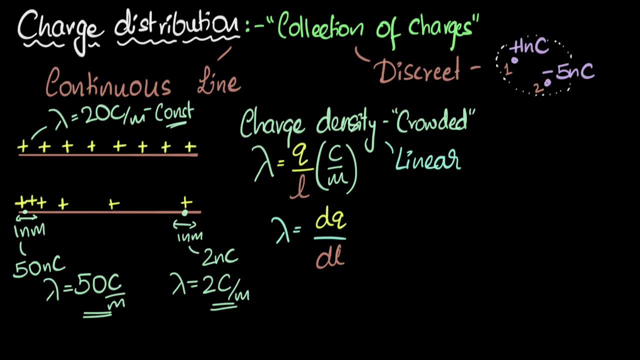 distributed over a line, over a meter, right. so this is one kind of charge distribution. are there other kinds of charge distributions? the answer is yes, and if you got this, then rest of it's very similar. so let me show you another kind. in fact there are three kinds. so the second one let me just write over here. 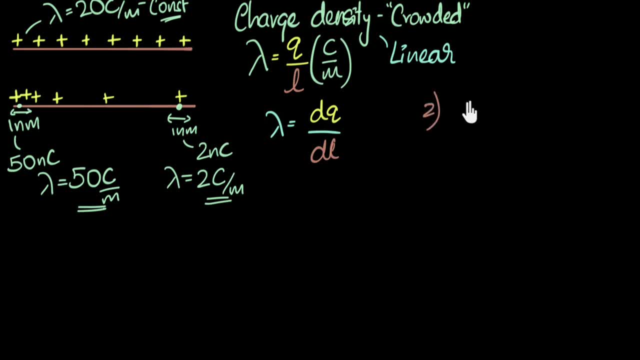 or let me do that over here, in fact, let me do that over here. second one would be surface charge distribution. surface charge distribution. and you can kind of kind of imagine just by looking at the word: now, instead of charges being distributed over a line, we have charges distributing over a surface. 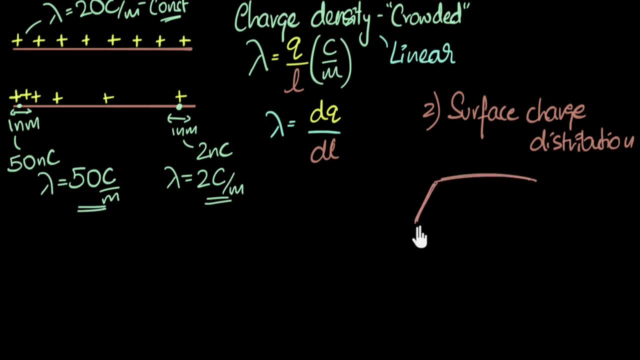 so you can imagine, let's say, this is some kind of a, I don't know, maybe a metallic plate. you can imagine this is surface of a balloon, whatever you want. and let's imagine now there is, there are charges everywhere on the surface and again it's continuous, the charges everywhere. this is what we call a. 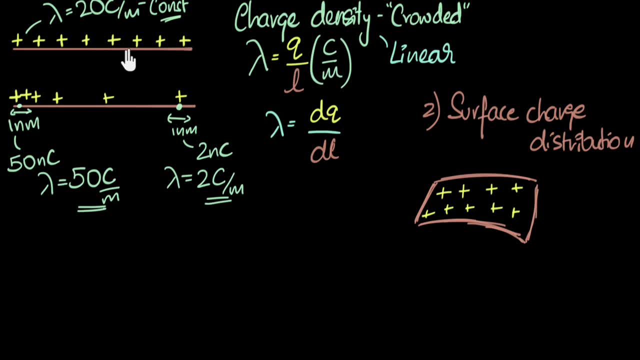 surface charge distribution and we have the same nuances, like we saw over here. you could either have distributions, which is uniform, so the density would be the same everywhere, or you would have non uniform. but my question is, how would you define charge density here? here it was charged. 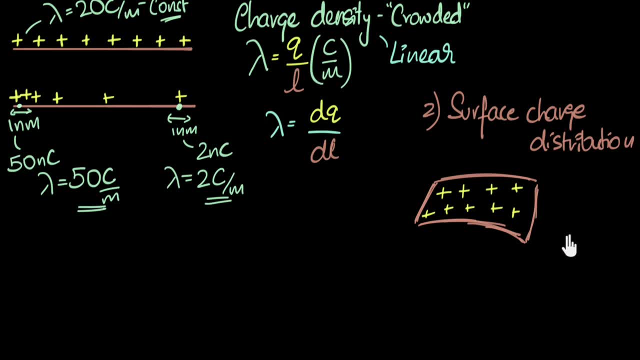 per length, coulomb per meter, what would we be over here? what would be the units? can you pause and think about it? well, over here, since we had charges are distributing over in area, here we introduce surface charge density and the symbol we use here is the voltage density. so if we have the charge density over the surface charge density and the symbol we use here 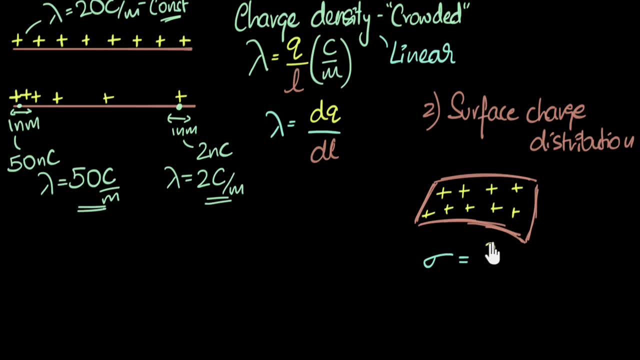 is sigma and surface charge density is just charge divided by area. So the unit over here would be coulomb per meter square. So, for example, if I said this was a uniform charge distribution and let's say sigma is, I don't know, maybe 10 coulomb per meter square, What am I saying? What? 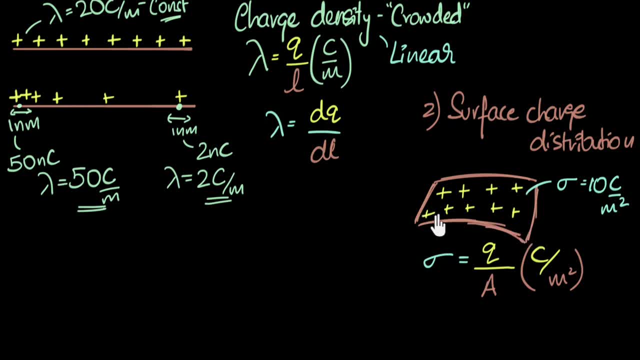 is the meaning of that? It means if I go anywhere on this surface and if I take, let's say, one meter square area, I'll find 10 coulombs of charge on it. But if I take two meter square area, then I'll 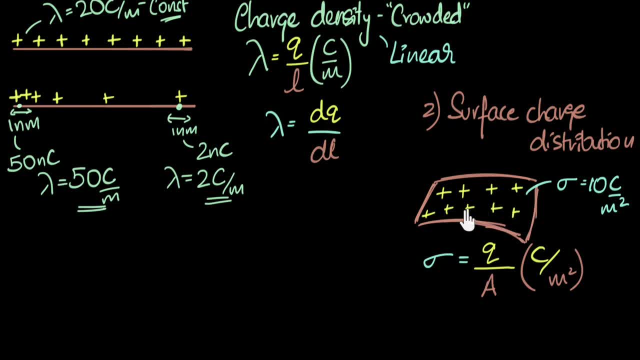 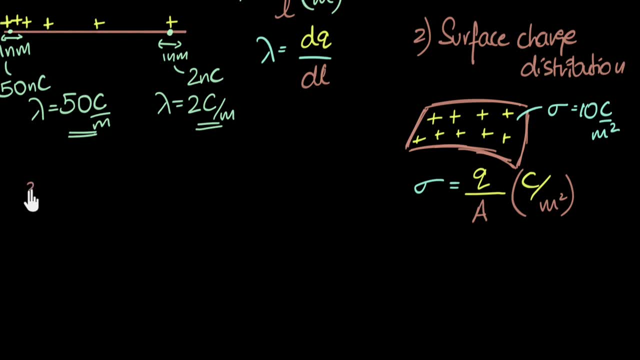 find 20 coulombs of charge on it and so on and so forth. And lastly the third and the final kind of charge distribution. I'm just like I've not arranged this very nicely, but the third kind would be volume charge distribution And again, I'm pretty sure you can kind of guess what this is. 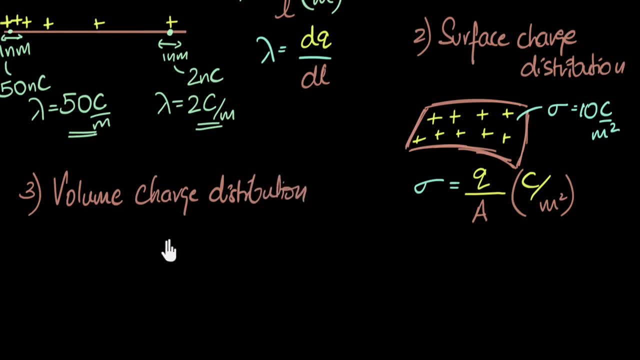 Now charges are distributed. charges are distributed by the volume of charge. So if I take a charge distribution, I'm just like I'm just distributing in space, in 3D space. So you can kind of imagine, let's say there's a box, Let me. 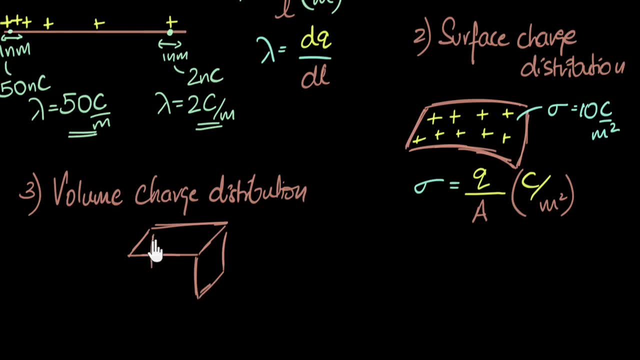 draw a cube type. a cube over here, a cuboid over here. Maybe this is my room. Yeah, my room is cuboid, I think. Okay, Anyways, now imagine there are charges everywhere inside in 3D space. 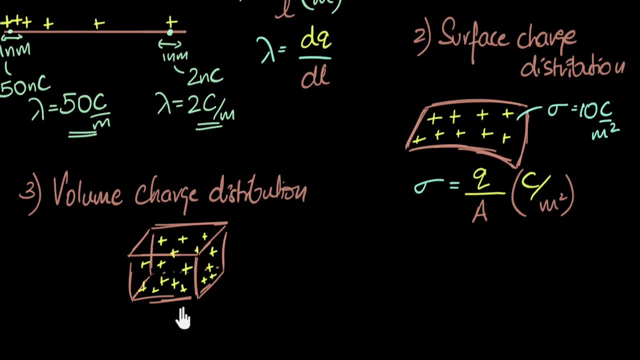 This is volume charge distribution, And exactly the same thing holds here. You can either have uniform charge, you know charges uniformly distributed over a volume, or you can have them non-uniformly distributed over volume. And again the question is: how do you define a charge density? 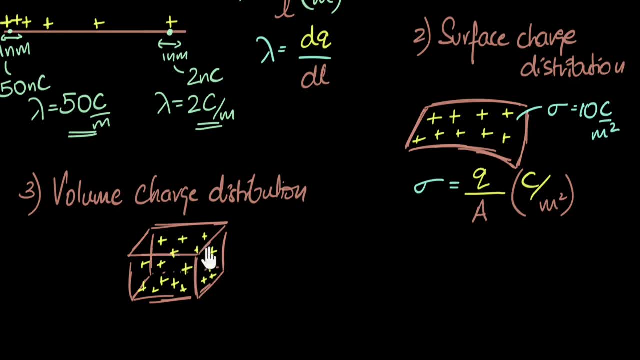 over here, Can you think? Well, since it's spread over a space, here we define charge density as, and the symbol we use is rho. I think these symbols are something you need to remember, But the way we define it over here would be charge per volume. 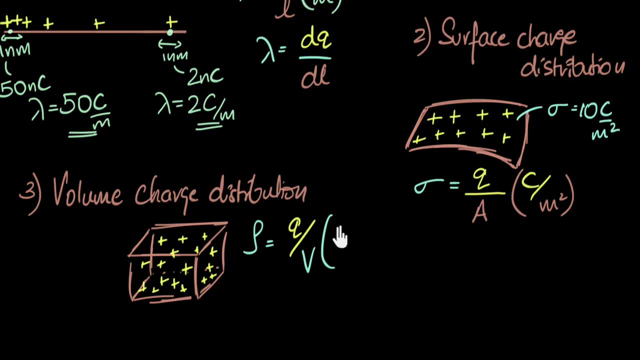 And the units would be coulomb per meter cubed And just like before, if you're dealing with non-uniform charge distribution, then you have to do dq over dv. At every point you would have different volume charge distributions. So let's put it all together. Let's put this all in one. 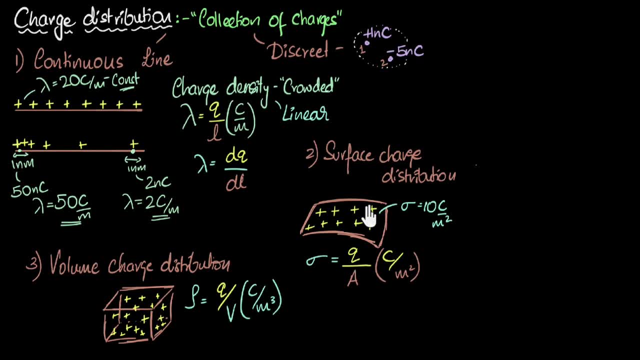 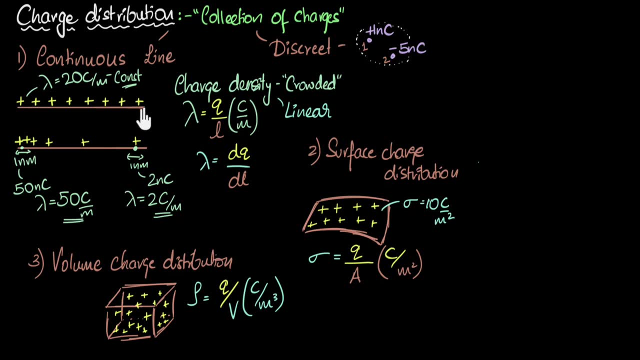 screen. Let me All right. So if you put it all together, continuous charge distribution is continuously. you can have them spread out over a line or a surface or over a volume, And one of the most important quantities is charge density. It tells you how crowded charges are distributed. 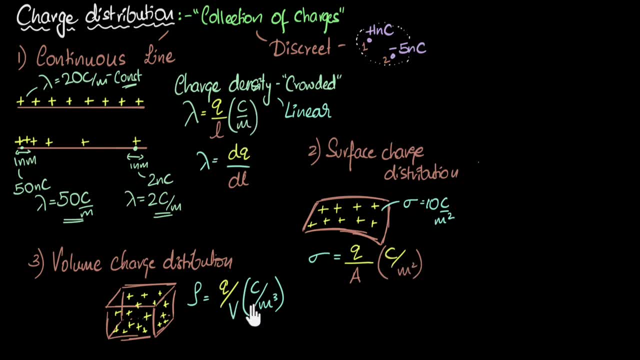 over a line, over a surface or over volume. If the value is a constant, which is my favorite, then that means it's a uniform distribution. If the value is not constant- it changes at different, different points- then you'll have to use differential differentiations. Then it means 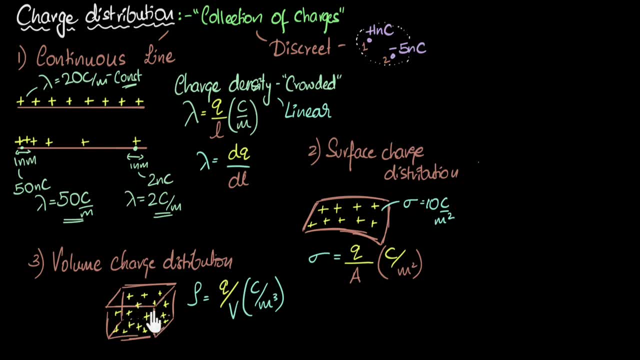 that charge density, charge, distribution, it's not uniform, it's varying. At some points you have more crowdedness compared to some other points.